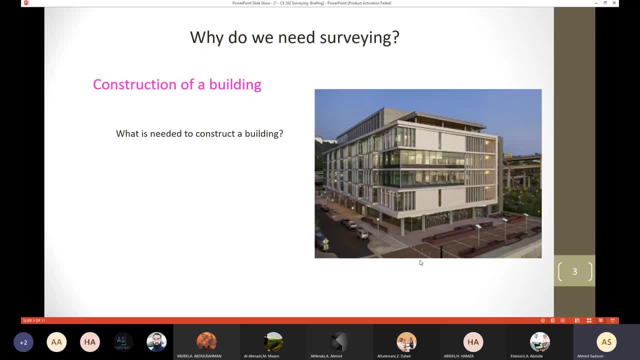 So let's say that I want to construct a building for a certain setting. So what is needed to construct a building? Before construction of the building, I need to know the site selection. I need to select a certain site. okay, a certain area. 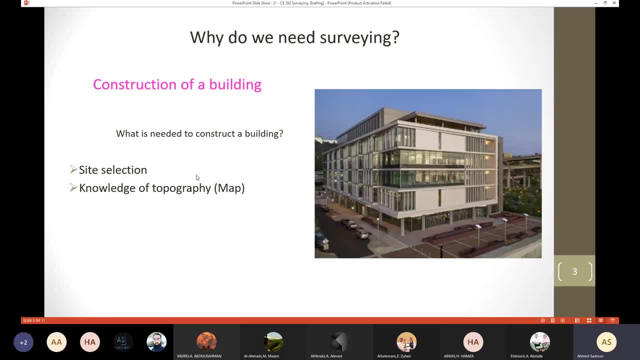 Then I need to know the topography of that area. Through the topography I'm going to know the elevation of that area. Maybe the site is located on a mountain, okay, or any other condition. So I need to know the topography. 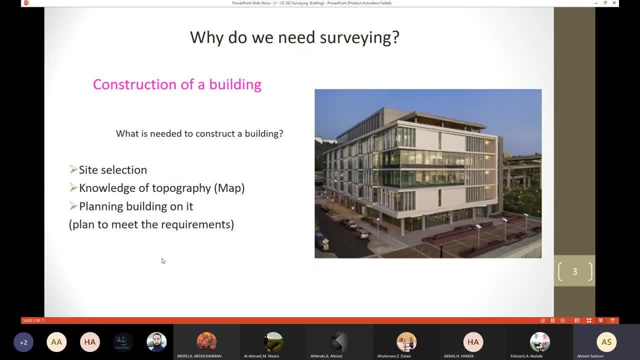 So that I know the nature of the site. Then, after I know the site and I know the map, the topography of the site, I will be able to make the planning. Okay, so I'm going to plan in order to construct that building. 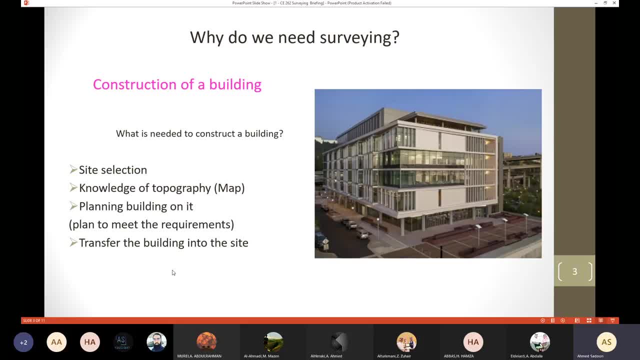 And the plan should meet the requirement. So now I need to transfer the building into the site. Now I draw everything. The architect Imagine the building, Draw the floor and the sections and everything, And then it has been delivered to the structural engineer or civil engineer. 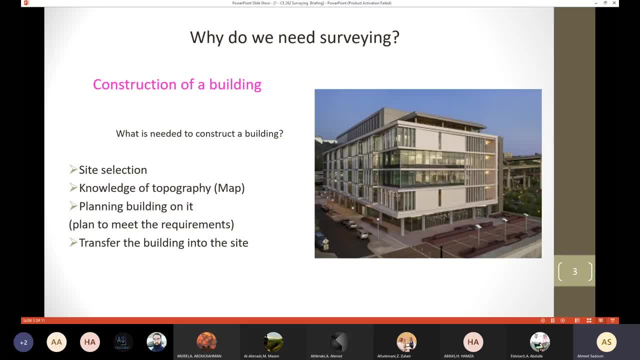 Also, he has done his job Okay. he drew the foundations, He drew the beams, the columns, everything. But everything now is on the paper. We need to transfer the design to be assigned. So how we are going to do that. 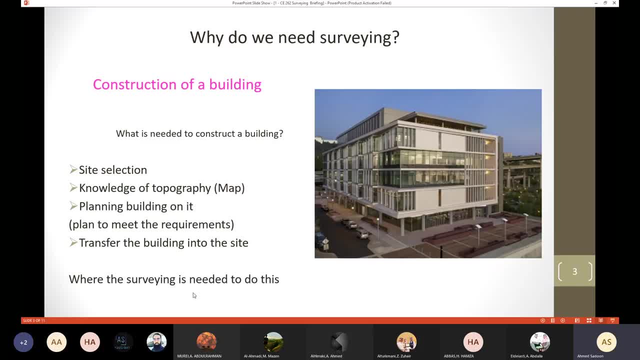 This is where the surveying is needed to be used. okay, So that there is a surveying, I'm going to transfer what we, what would have been written or what would have been designed. I'm going to transfer this on into the site. 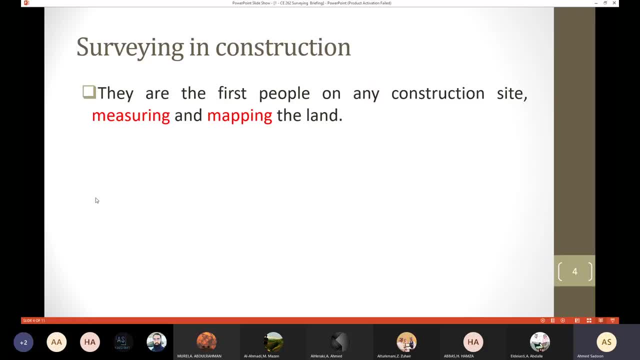 Okay, So in the surveying in construction- they are the first people on any construction site. They are going to make the measurement and the mapping of the site- Okay, the mapping of the land as well. these primary measurements are then used by the architects. 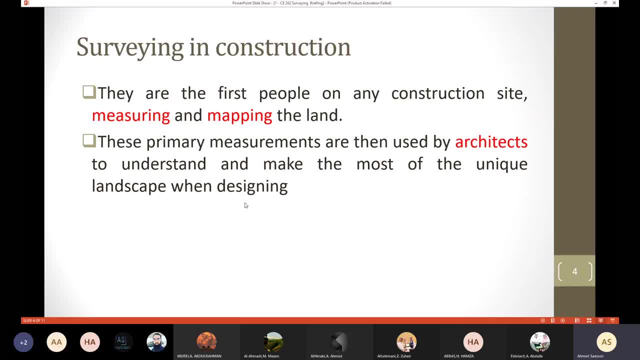 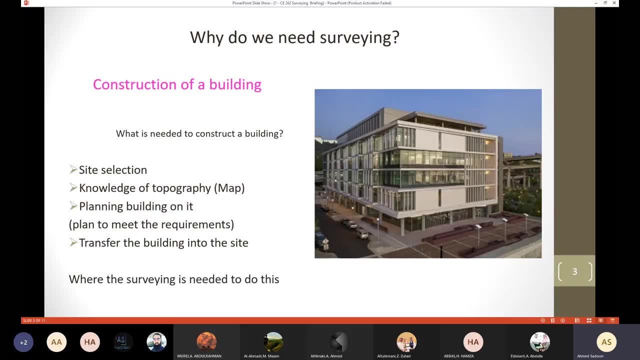 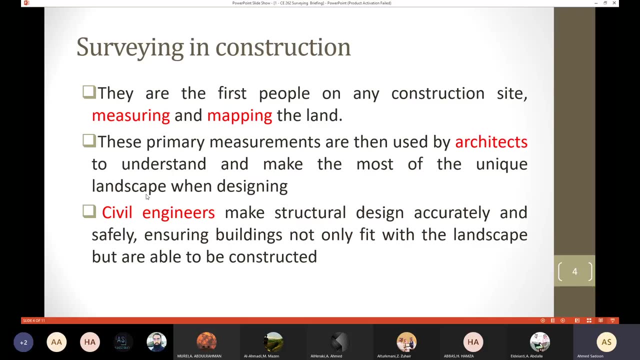 to understand and make the most of the unique landscape. one design so without here, without the knowledge of the topography which is the map is going to be drawn by the surveyors, the architect will not be able to make his design. okay, then the civil engineers make structural design. 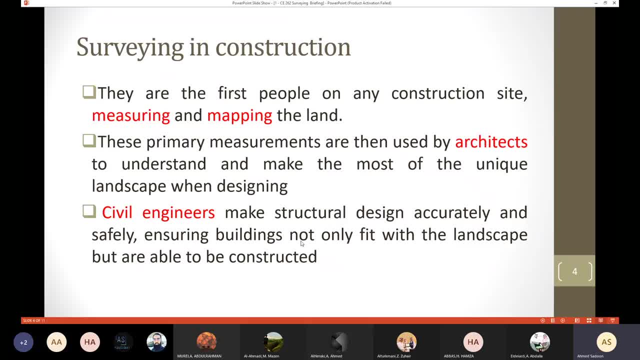 accurately and safely, ensuring buildings not only fit with the landscape but are also able to be constructed okay. so the surveying is very important for the architects so that they know the landscape, and also it's very important for the civil engineers so that they are going to transfer. 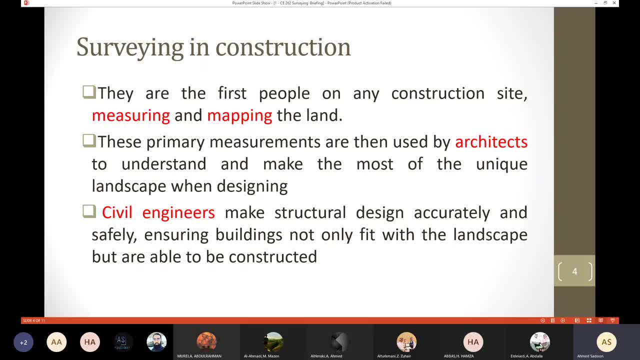 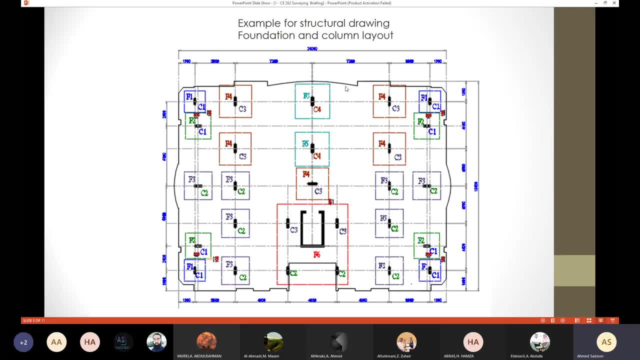 what would have been designed to be assigned on the site. so, for example, let's say, here we have a structural drawing for foundation and column layout. here i have foundation and i have columns. okay, i think most of you took autocad, so you are familiar with this kind of drawing, okay. so 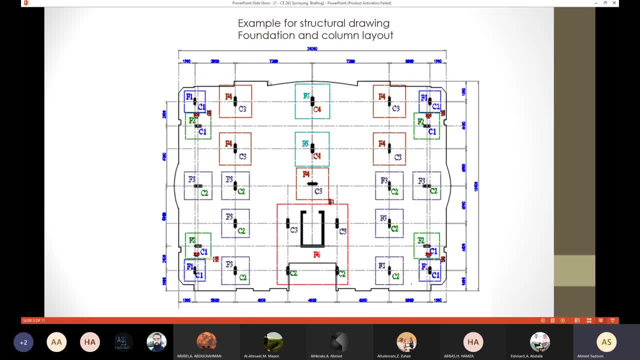 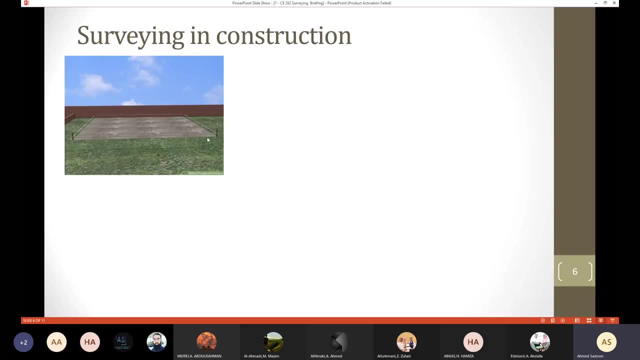 this has been designed by the structural engineer. now i need, i need to transfer all of this drawing to be uh, to be done on the actual site. so i need to make, i need to know the corners of the site, which the process should be done by the surveyor. he know how to measure all of this. 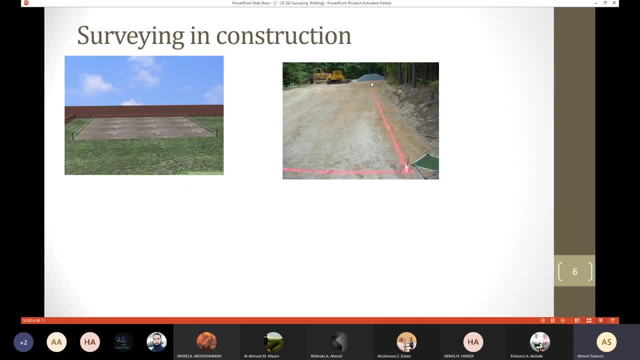 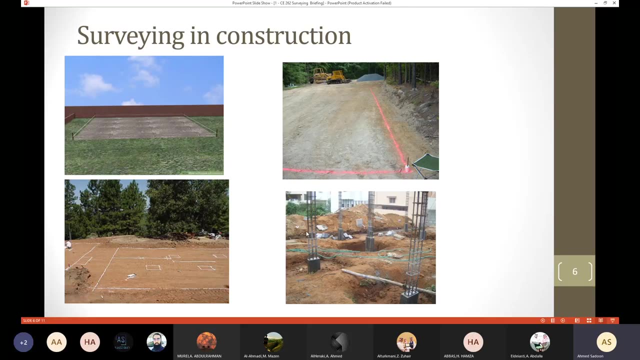 he know how to locate the corners of the site, then he are going to draw it like that on the side, then he are going to precisely locate the position of the foundations- okay, and then i'm going to be able to cast the foundation and the column okay. so let's say that. 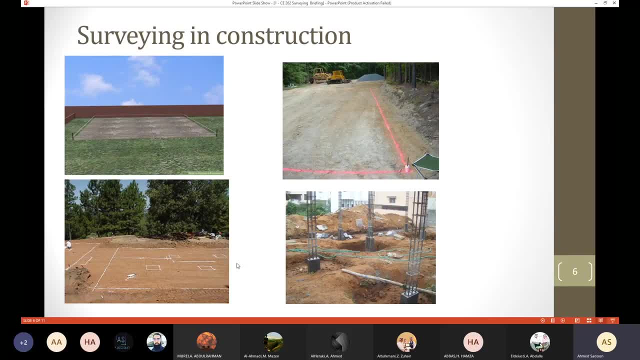 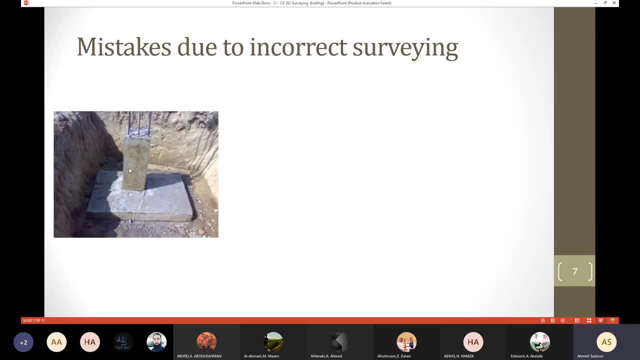 uh, all of this work has not has not been done. precisely what will happen? we are going to have problems like this. like you can see that here we have lousy job. the column is not in the center of the foundations because of the poor measurement. so through the survey we will be able to precisely. 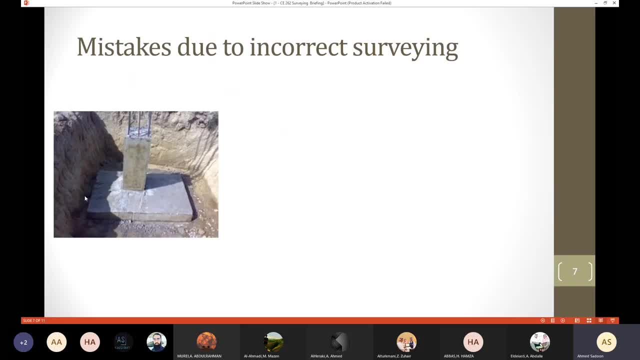 put all of this in the uh, in the wanted places, otherwise you are going to have problems like that also. in order to bridge, uh, to build a bridge or construct a bridge, we are not going to start from one side, because if you are going to start from one side, the project is going to take a lot of time. so we 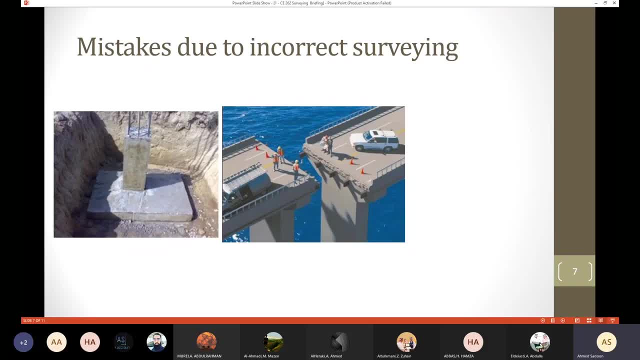 are going to start from the both side and the measurement should be correct. the leveling, the location, the position, everything should be, uh, correct and precise, okay. otherwise we are going to have a problem like that: the, uh, the. the bridge is not going to be connected at the midpoint, okay. 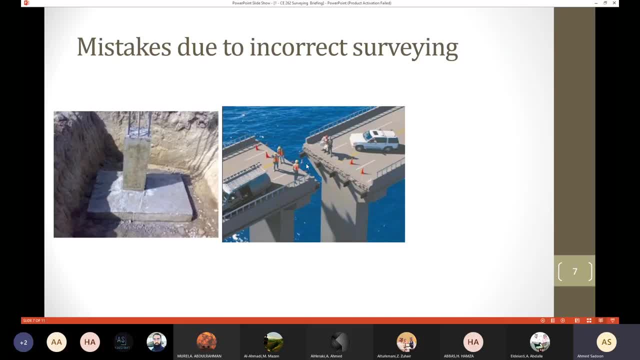 so if we have done lousy job, uh, in surveying, we are going to have problems like that also. you can have also problem like that. the column is not, uh, in a line with the other columns here. okay, so if the surveying job has not been done precisely, we are going to have problems like this. so surveying. 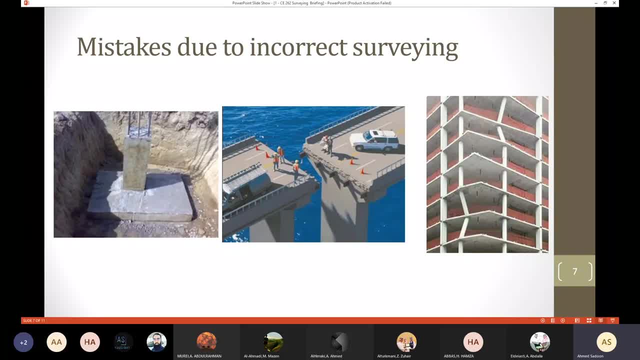 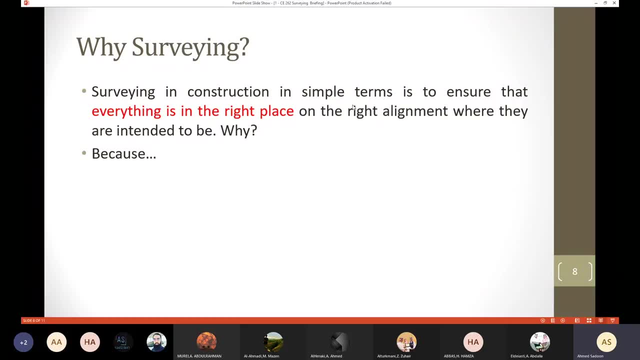 is about measurement: measurement distances, measurement angles, measurement positions. so why we need surveying? again, surveying is a major μεły cель swap. so when we have any survey subject construction, in simple terms, is to ensure that everything is in the right place. So in simple, 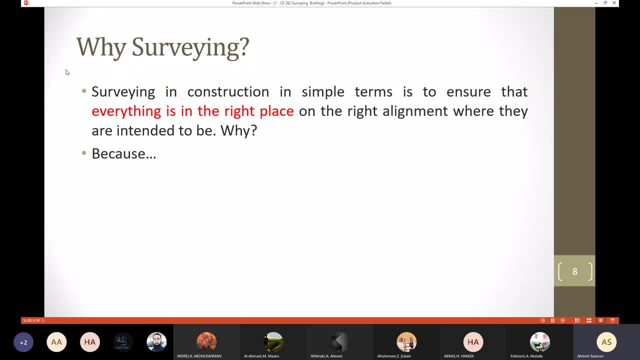 words. surveying has been existed to make sure that everything is in the right place, on the right alignment, where they are intended to be. Why? Because we don't want conflict, especially in property line. You are familiar with the property line, the line between you and your. 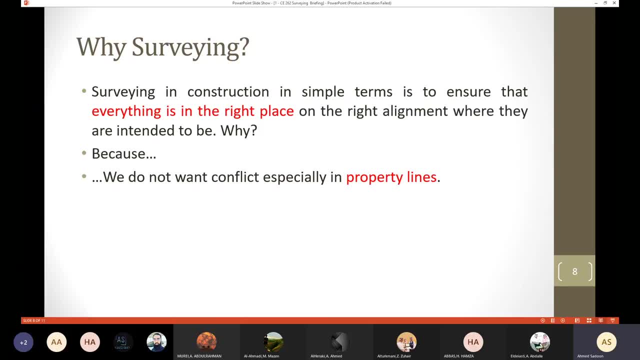 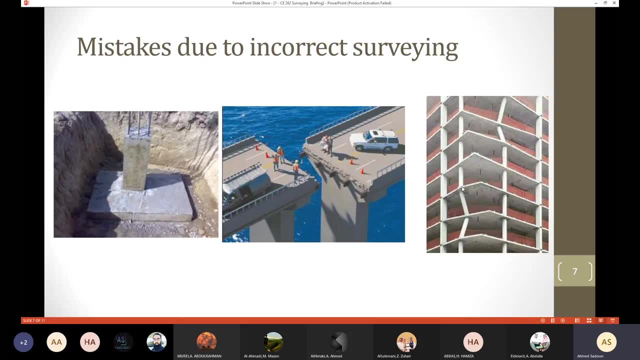 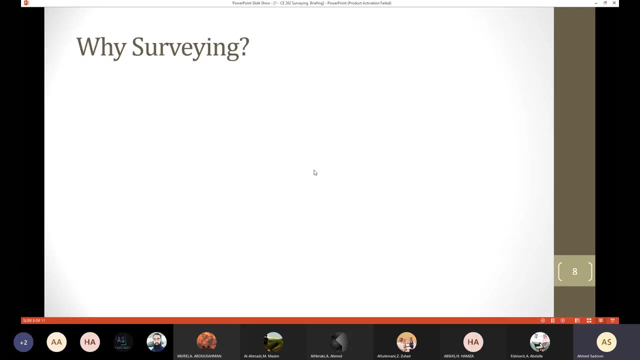 neighbor. So if we have poor measurements, then we are going to have a conflict with your neighbors. Also, we don't want unblumped columns like this one here, Okay. Also, we don't want to have misaligned structure like this one here, Okay. So we want the elevation to be corrected. 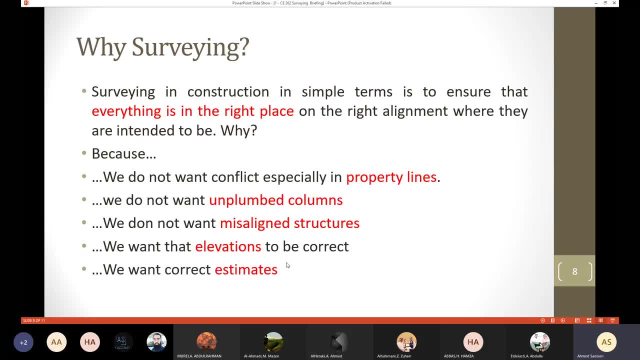 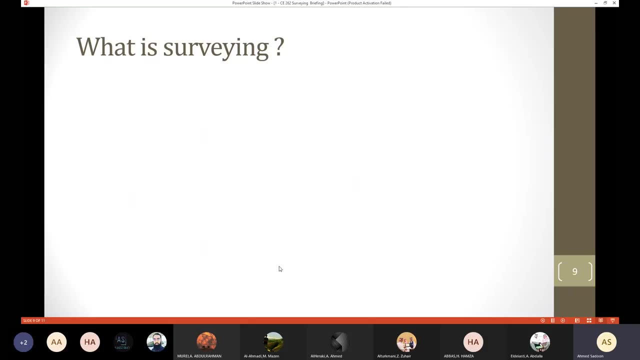 We want to have correct estimates. We know that estimation is very important for many jobs, in order to know the cost and many other things. So without the surveying, all of this would not be possible. So again, what is surveying? Surveying is the art and the science. 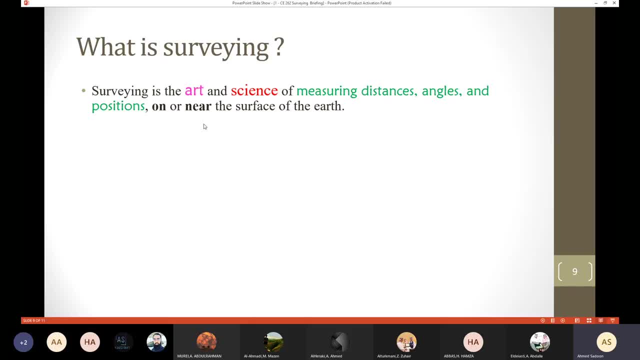 of measuring distances, angles and position on or near the surface of the earth. So is it an art- Surveying? do you consider surveying to be an art? Yes, Because only a surveyor who has a full understanding of surveying techniques. 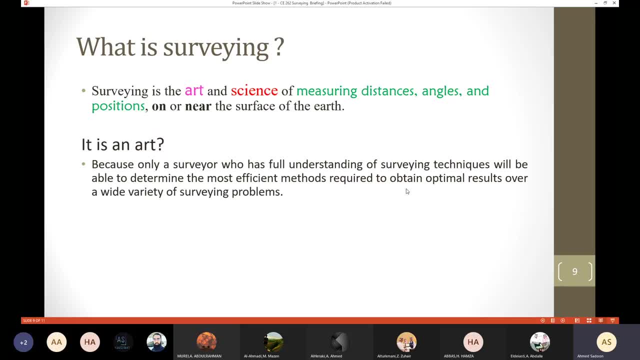 will be able to determine the most efficient methods required to obtain optimal results over a wide variety of surveying problems. We have a lot of problems. We have a lot of methods. Only the surveyor who has a full understanding will be able to choose the best method to the job. 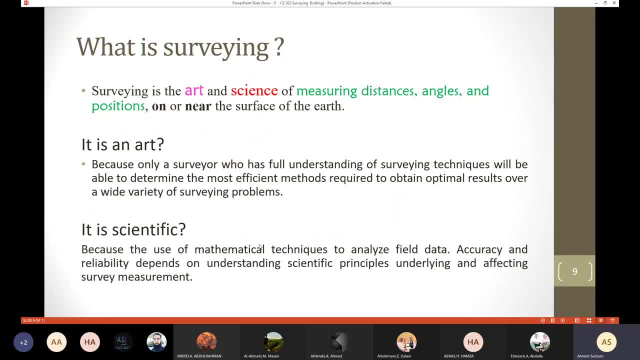 Is it scientific? Yes, it's scientific because we are going to use mathematical techniques to analyze the field data. Okay, So the accuracy and the reliability depends on the understanding of the scientific principles. So surveying is an art and it's a science of. 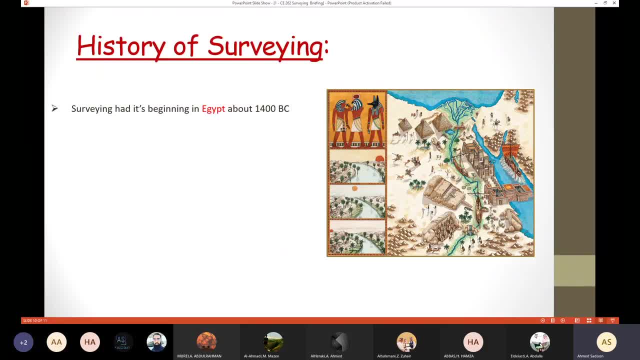 measuring. We know, we need to know that surveying it has a long, a long history, Okay, Very long history, Okay. So surveying had its beginning in Egypt about 1400 BC, mainly because the land along the river, the Nile river- here we have a Nile river And at that time 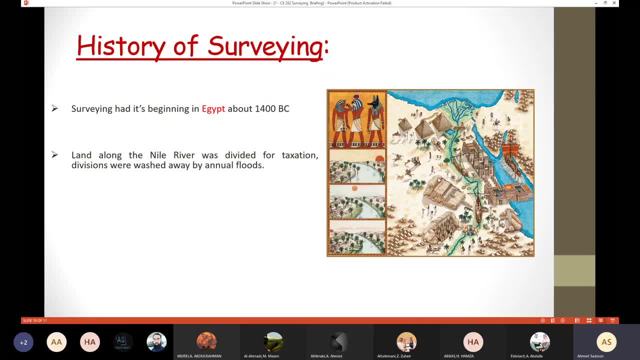 the people live around the river here because we have water, we have the green land, So people at that era live around the river And their land and their houses is going to be located here. But we have a problem with the Nile river. At a certain season the river Nile is going to flood. 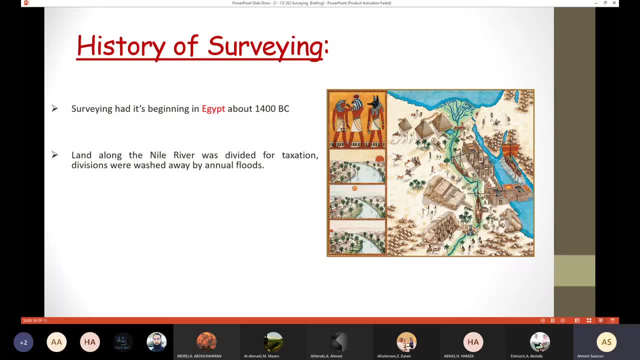 Okay, So after the flooding we are going to, we are not be able to precisely to know the the location of the lands for the people And at that time they have. they used to have a taxation system. They are going to charge you with the money for what you are going to own. Okay, So, 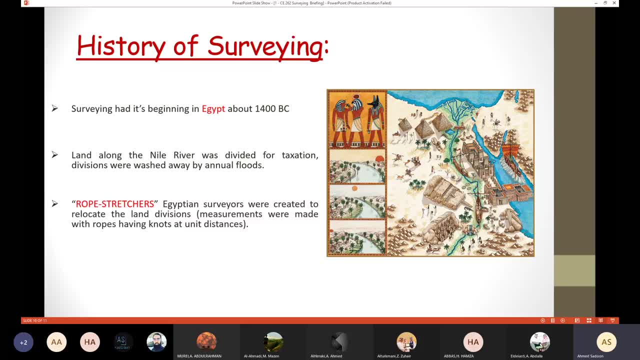 that make problems for them. So what they do, we have Egyptian surveyors. At that time they called us. they can compute road規. they can study road規. We don't have it today, but it is casual. So the elections 2020, we're going to be spending time to see how the election is going to adjust. 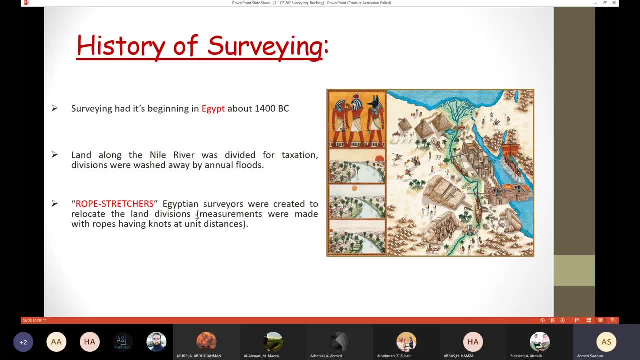 the characteristics of this system. Okay, I want to let you know, or the good news is that a lot of people have arrived, There's very little crowd and there's very few approximately, to all nicely priced, 1960s, 27th century style, all year old. That's why we decided to do this. various kind of 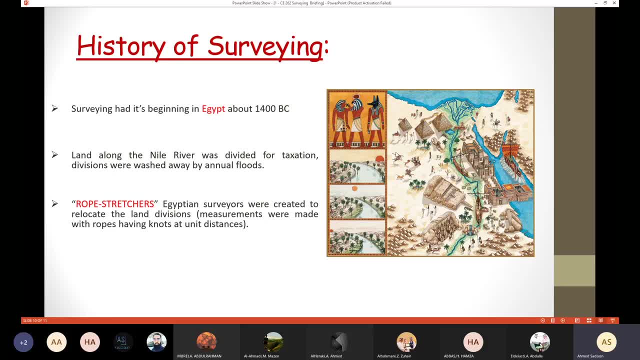 nuclear에요 and nuclear SpaceX project applied to us to inform our students a little bit, And then, therefore, we came to Main City. mom said that not only the earth, we were most concerned about the locations, and also we know that in that era we have a lot of monuments and in order to build,